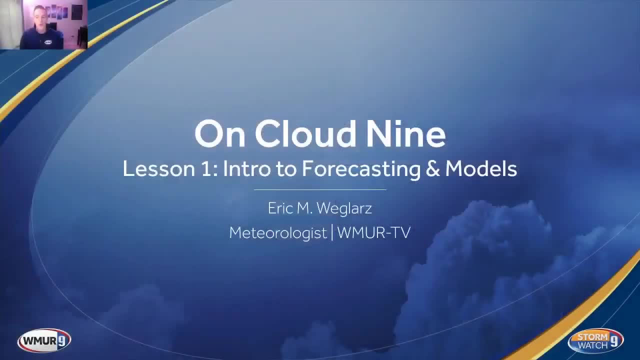 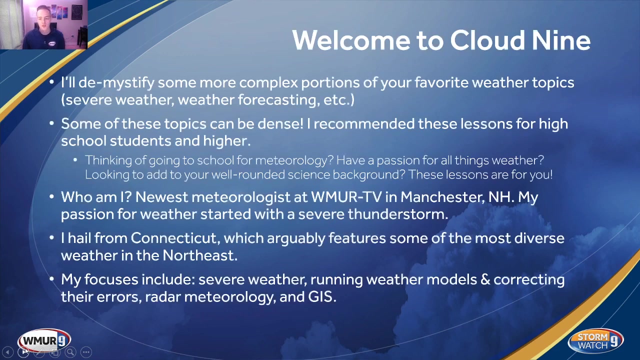 complex meteorology can be So welcome to. On Cloud Nine, That's what I'll be naming my segments- a play on the phrase there- And the first segment that I figured I would do with everybody here will be an introduction to weather forecasting and weather modeling, which is also known as 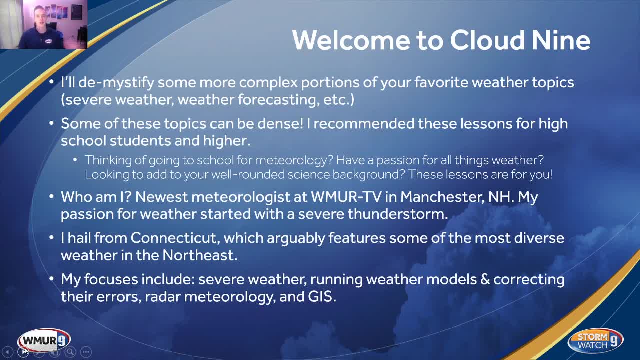 numerical weather prediction. So, as a broad overview, I will hopefully attempt to demonstrate some of the things that I'm going to be doing in this segment, And I'm going to mystify some of the more complex portions of your favorite weather topics, which might include: 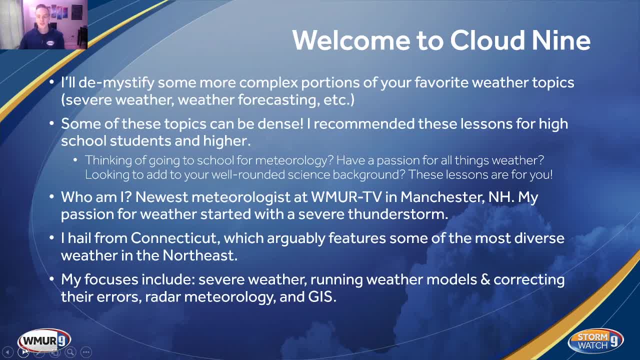 severe weather, winter weather, weather forecasting, things like that, And a number of these topics, like I mentioned, are dense, So I recommend that these lessons are viewed by high school students and higher, especially those thinking of going to school for meteorology. 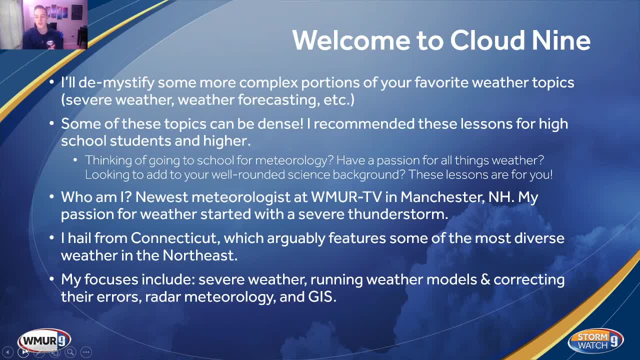 They have a passion for all things weather And maybe you're looking to add to your already well-rounded science background, then these courses will certainly be for you. I am the newest meteorologist here at WMUR-TV in Manchester, New Hampshire, And, like so many, 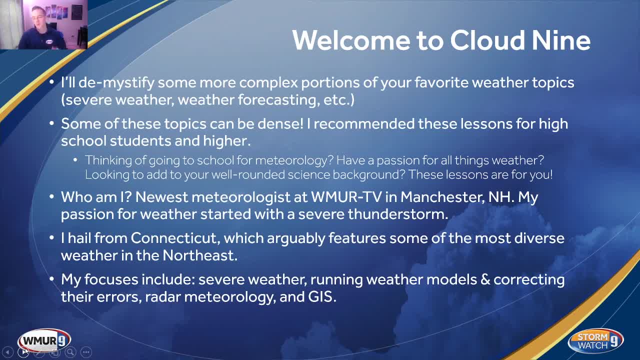 meteorologists, our passion for weather started with a particular event or series of events. It might happen to be a severe thunderstorm when I was, I think, nine or 10.. So, boy, do I feel old. But way, way back when I was young, I saw the most vivid thunderstorm I've ever seen, And that 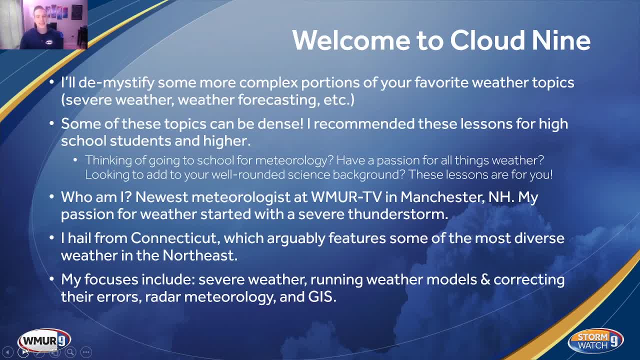 really fueled my passion to where I am now. I also hail from Connecticut, which arguably features some of the most diverse weather. I'm going to be talking about some of the most diverse weather across all of the Northeast. We have severe weather, winter weather, We have nor'easters. 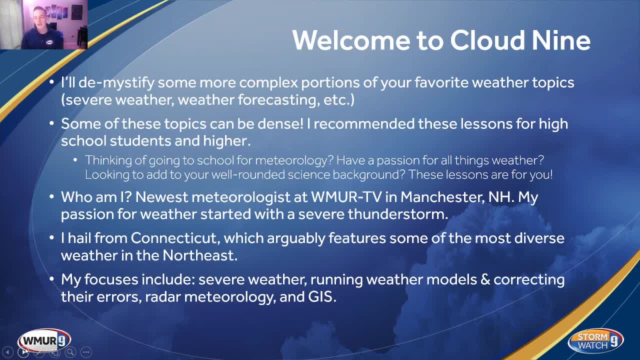 blizzards, We have extreme heat, extreme cold, We have flash floods, You name it, we have it, And that really was the catalyst for where I am today, And my focuses include severe weather. no surprise there, running weather models and correcting their errors, radar meteorology. 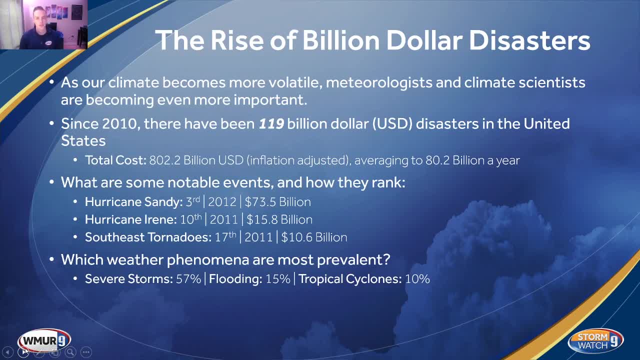 and GIS, which is short for Geographic Information System. So before we get into the weather forecasting piece of this presentation, I figured I would start off with talking about the rise of billion-dollar disasters. So, as you've seen in some of Haley's prior videos, our climate is certainly changing around and is changing around, unfortunately. 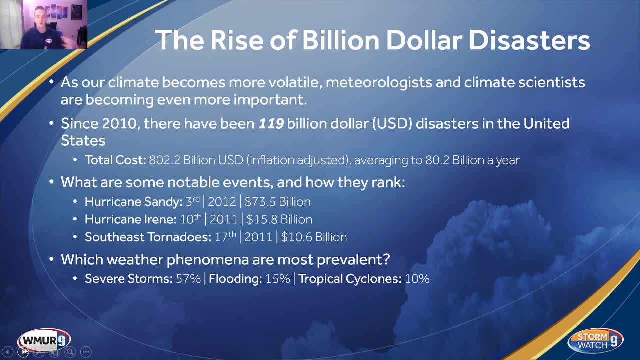 to the more volatile part. So weather is becoming more volatile and is becoming more destructive, So the role and the importance of meteorologists and climate scientists is becoming even more important. There's no doubt about it. So I'm going to be talking about the rise of billion-dollar. 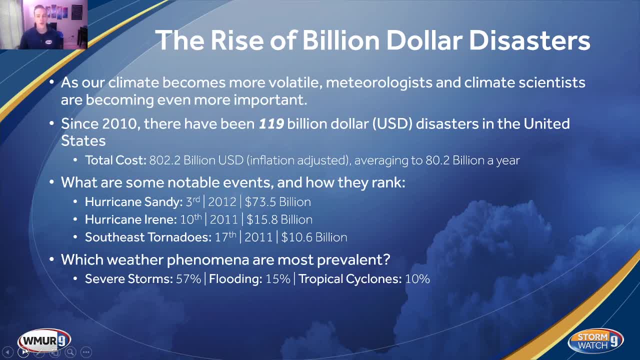 disasters. So before we get into the weather forecasting piece of this presentation, I figured I would talk about that. And since 2010, there have been 119 individual billion-dollar disasters in the United States. So this is a weather phenomena or a series of phenomena at one particular event. 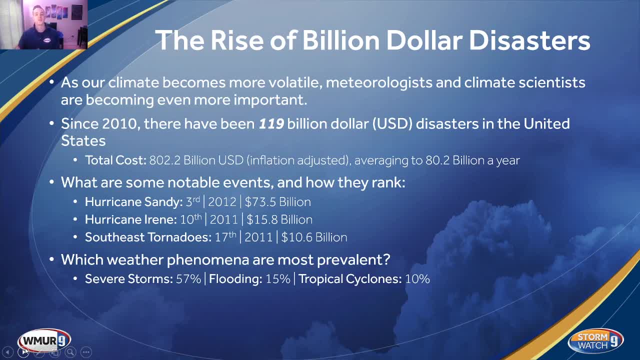 that add up to a billion dollars or more of damage, So the total cost of all of these disasters comes out to $802 billion. We of course, account for inflation in this, which averages to $80 billion a year. Think about that Weather. 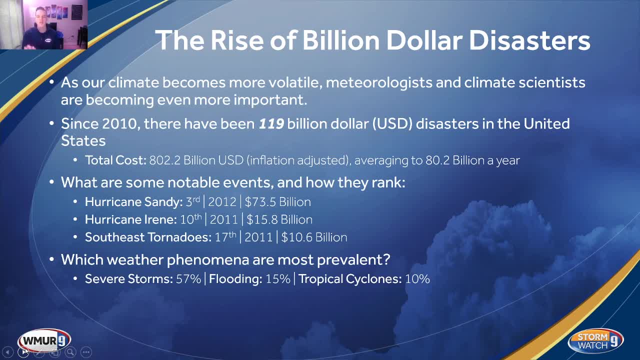 destructive weather creates $80.2 billion of damage a year. It's impressive to think about the power of weather, but how more powerful weather has become compared to what we saw maybe 40 or 50 years ago. Now there have been destructive events in those years, but the frequency of those 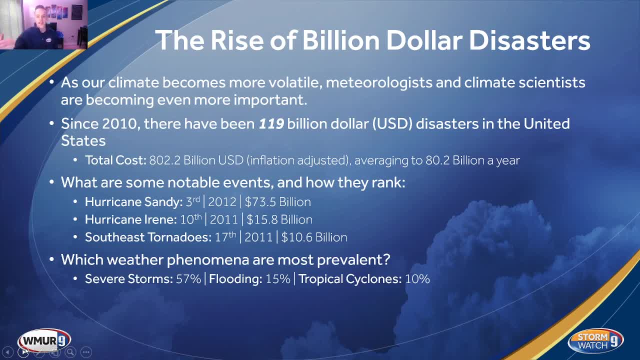 events one could argue has certainly increased over time. Now, what are some notable events and how do they rank? Well, Sandy, for most people who remember this. third since 2010, with $73.5 billion worth of damage. So that's a lot of damage, That's a lot of damage. That's a lot of. 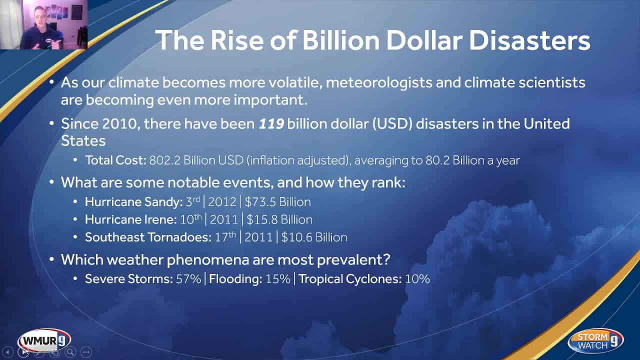 damage. So think about that. Sandy alone almost accounted for an entire year's worth of damage just from that one tropical cyclone, in this case extra tropical Hurricane. Irene came in at 10th in 2011,- just a year prior, and the Southeast super outbreak of severe weather especially. 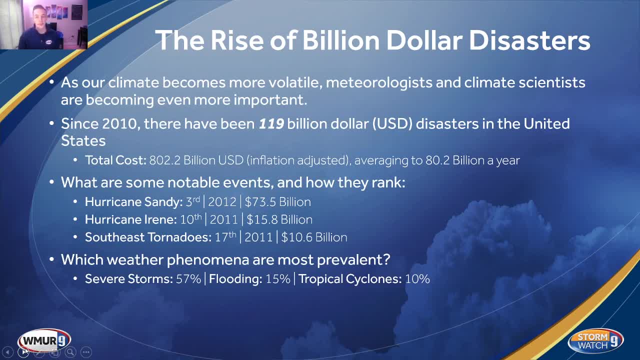 the tornado part in Alabama in 2011 as well, caused just over $10 billion of damage. So which weather phenomena are most prevalent in this entire breakdown? The thunderstorms, severe storms as a whole, no surprise- create just shy of 60% of the total. 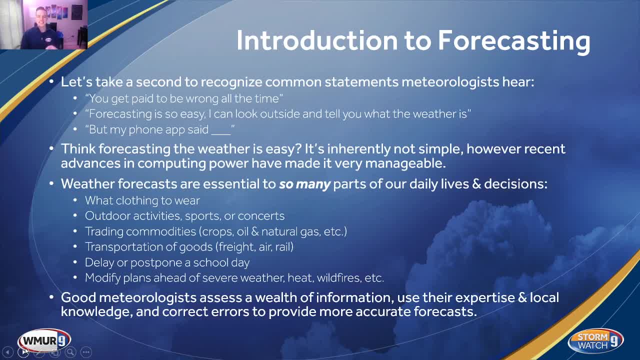 makeup, followed by flooding at 15 and tropical cyclones at 10.. So, with that in mind, let's go to the introduction to weather forecasting. So let's take a second to recognize a few of the common statements that meteorologists today hear, sometimes on a daily basis. You get paid to be. 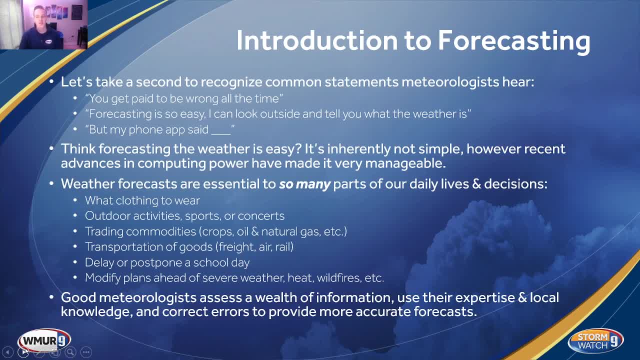 wrong all the time. That's my personal favorite. Forecasting is so easy. I can look outside up into the sky and tell you what the weather will be for the next few days. So let's take a look at some of these common statements that meteorologists today hear, sometimes on a daily basis. So let's take a second. 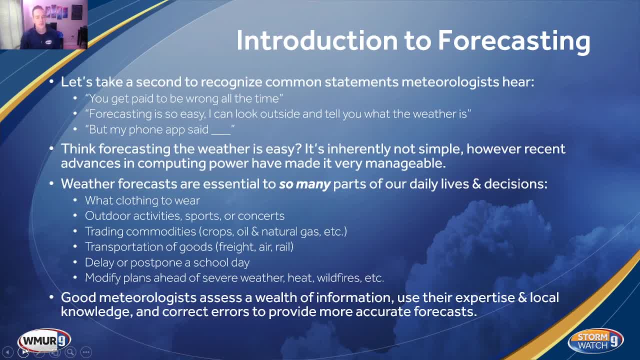 to recognize a few of the common statements that meteorologists today hear, sometimes on a daily basis. forecasting is so easy. Well, it's inherently not simple. However, recent advances in our computing power and uh research and technology today have allowed us to make it very manageable. 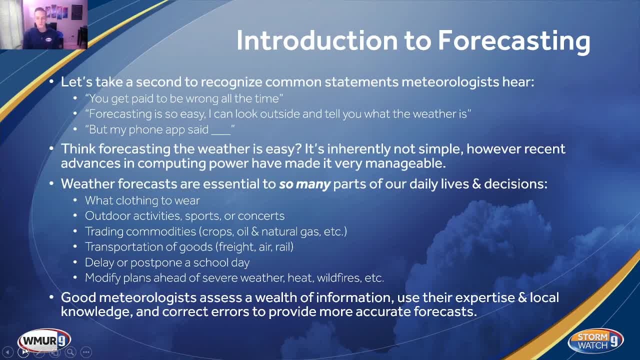 compared to, say, 40 or even 50 years ago. So think about it. When we think about forecasting, we think of it as a sort of a hypothetical formula. So let's take a look at a clue that. Think about this. weather forecasts are central to so many part of our daily lives and decisions. 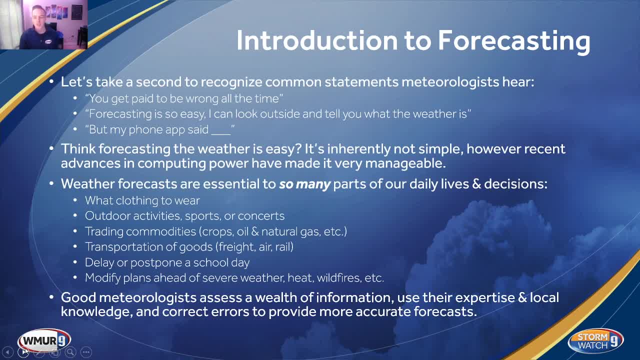 What clothing to wear. You're not going to wear a jacket if it's 85 degrees and humid. outside Outdoor activities, sports or concerts- severe weather can change those in an instant. NASCAR with rain. the races can't go on if the track is wet. 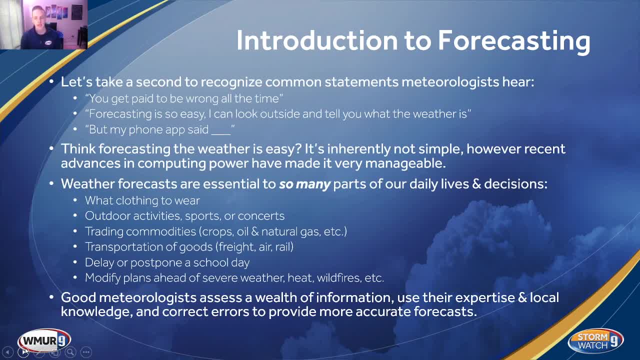 Trading commodities. if we are going to have a super cold outbreak, obviously we're going to need to purchase more in the way of oil and natural gas. That will certainly reflect on the stock market Marketing of goods freight air, rail superintendents needing to decide whether we're going to 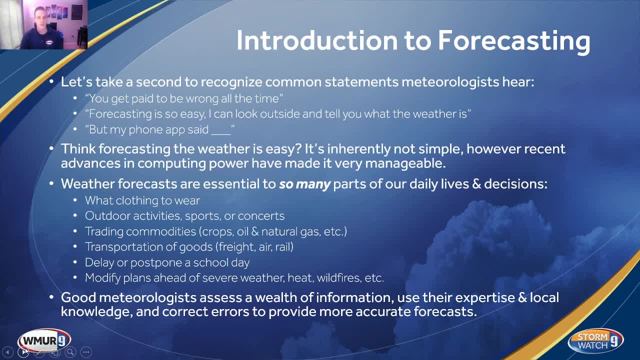 delay or postpone a school day based on a storm system coming in, how much snow falls, whether kids are going to or from school, will that impact those travels? whether we need to modify our plans ahead of severe weather, heat, wildfires in California- all of these 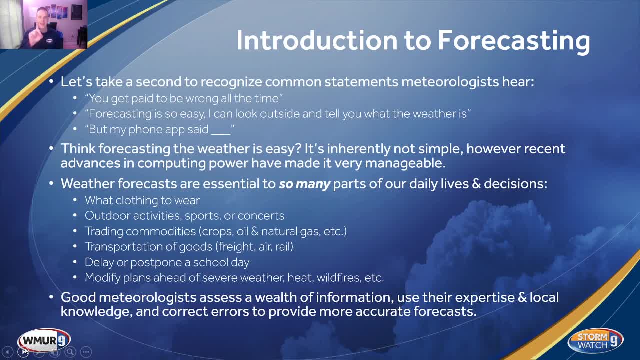 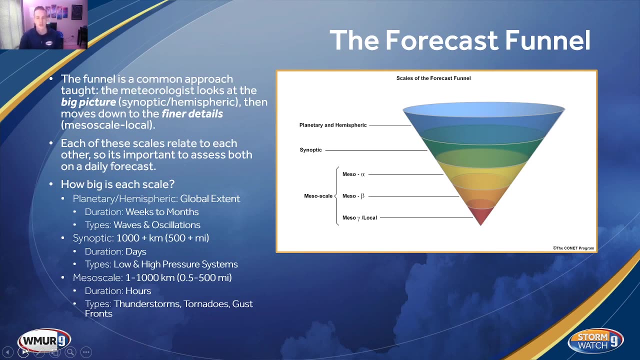 things rely on one thing in particular: an accurate weather forecast. So good meteorologists can assess a wealth of information, Use their expertise and local knowledge and correct errors to provide even more accurate forecasts with time. So the first approach, the first method we're taught when we're in college, learning about 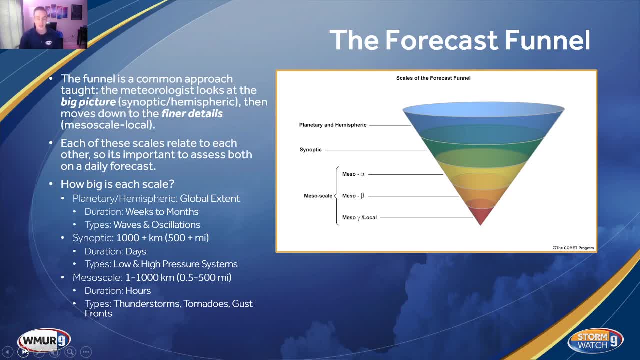 forecasting is one of the most common approaches that we use every single day and that is the forecast funnel. Simply put, the forecast. the meteorologist will look at the forecast, starting with the big picture, so the synoptic or the mesoscale, rather the hemispheric scale, and then go. 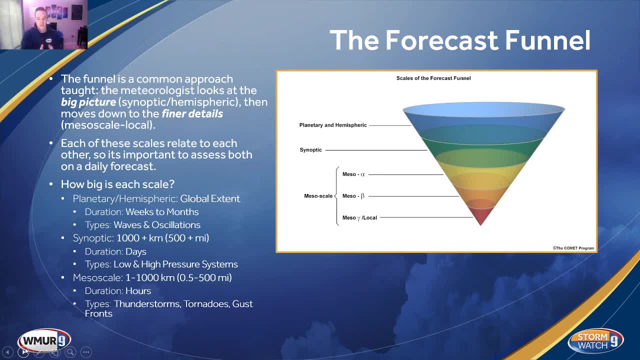 down to the finer details, which we will call the mesoscale: The mesoscale and then all the way down to the local scale forecast, which you most care about. Will I see rain at X location? How warm will it be? 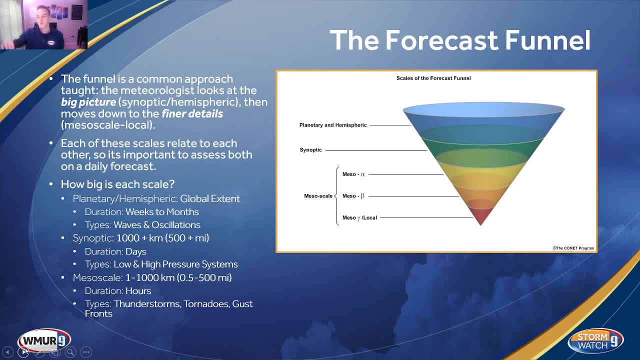 How cold will it be at this specific location? What's the chance of severe thunderstorms or 12 inches of snow at this particular location? You get that from the mesoscale, the fine scale details, And it's important to note that each of these scales relate to each other, so it's important. 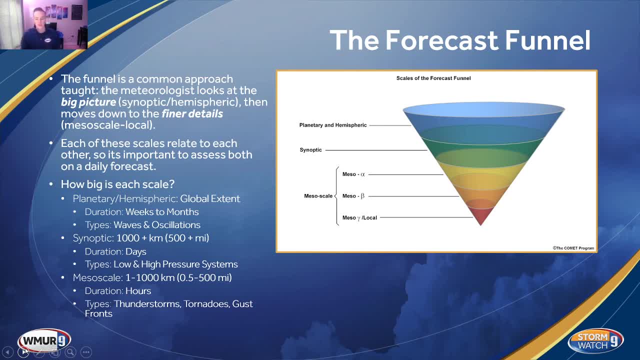 that we need to assess both, not just one or the other. So, of course, the next question is: what's the best weather forecast? You know a number of these scales. look- and I've never heard of this before- how big. 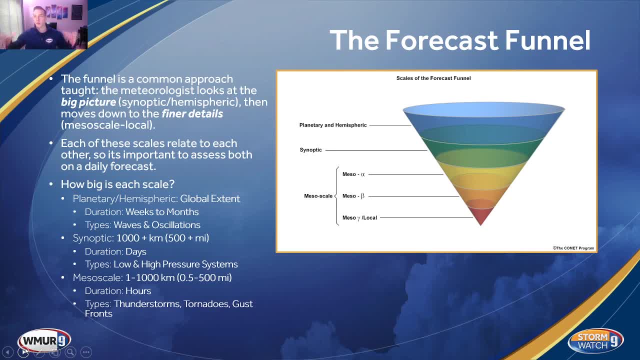 are they? Well, we start with planetary and hemispheric. We're talking about global extent. So, whether that be the continental United States, Europe, Asia, Africa, those make up the planetary and the hemispheric scale. So we're looking at waves of lows and high pressures and how those move along. 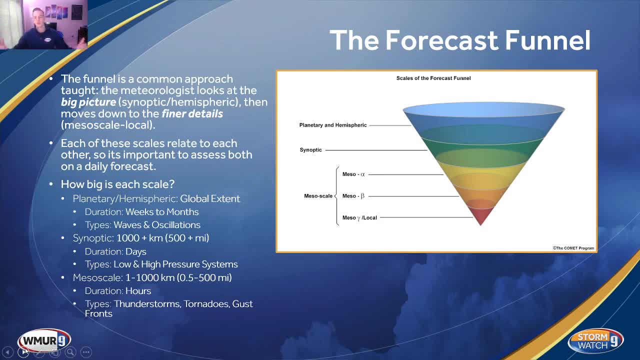 We're talking about big, big circulations and how those move over days and weeks. Next, the synoptic scale. So we measure things using the metric system in meteorology. However, for those folks who maybe aren't as familiar with the metric system, of course, 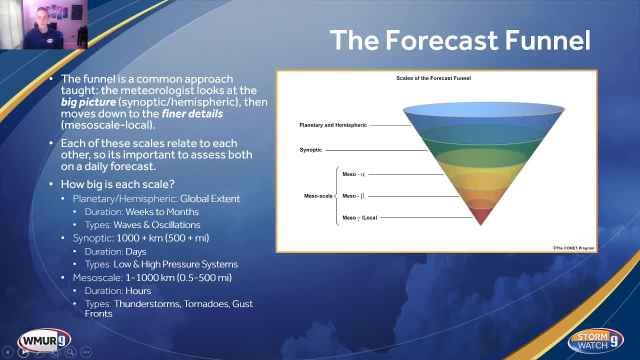 I included the conversion over to miles. So in this case we're looking at 1,000 kilometers plus, which is 500 miles or more for a length. We're looking at a duration of days And the types of weather. we look at this particular scale and the synoptic scale will, of course. 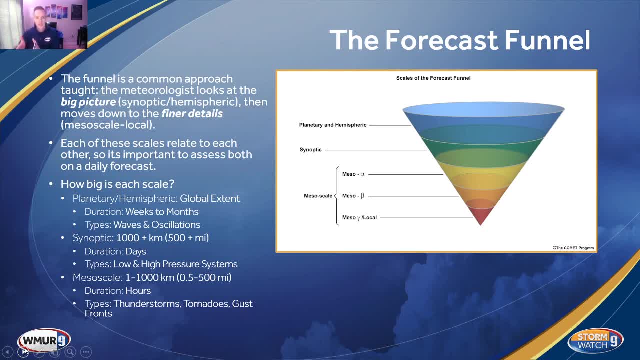 be areas of high and low pressure and how they move with time. Next we go to the mesoscale, so 1 to 1,000 kilometers, which adds up to a half mile, to 500 miles, potentially a little bit larger. 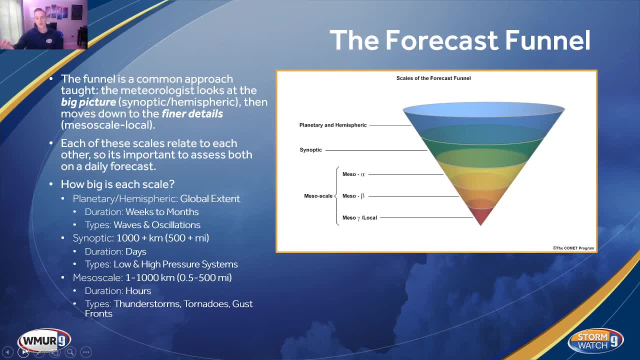 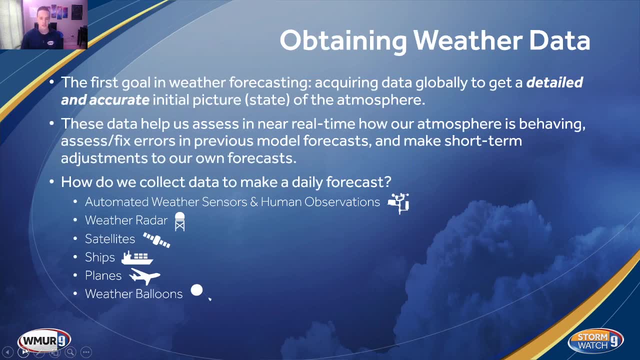 And the duration of the weather phenomena in this scale- usually lasts a couple of hours at most- And the types of weather we see- thunderstorms, tornadoes and gust fronts- and how those interact and, of course, how long they last. So the first thing we need to do as a good meteorologist, or as good meteorologists, is: 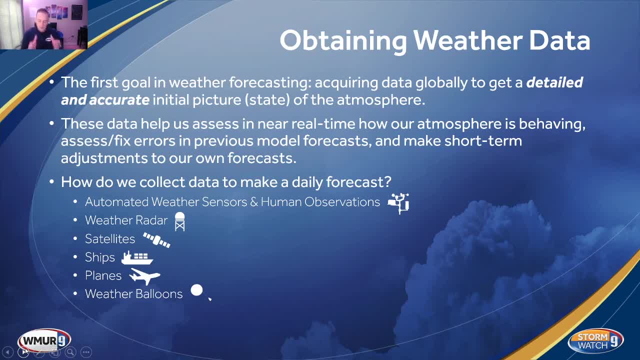 obtain data globally- not just in one particular location, but globally- To get a detailed and accurate initial picture or state of the atmosphere. Our atmosphere is a fluid And in order for us to get a good idea as to what's going on with the entire atmosphere, 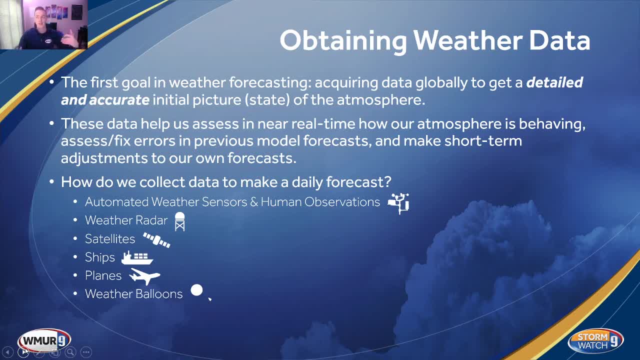 a highly movable and volatile fluid. in some cases, we have to get a very detailed picture, as best we can, of the entire fluid across the entire globe. Think of it as like a bathtub more than anything else. So these data help us assess how our atmosphere is behaving. 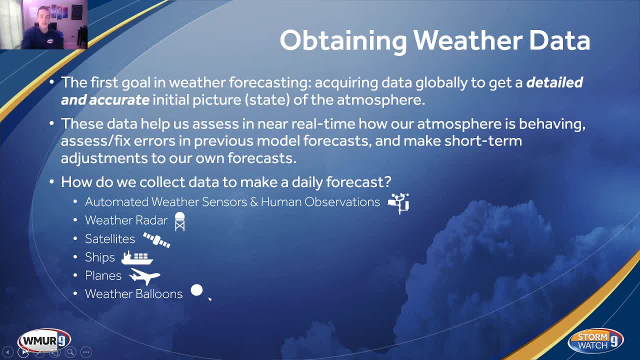 We can assess and fix errors in our previous forecasts And previous model forecasts and make short term adjustments to our forecasts we've made in the past. So the next big question will, of course, be: how do we collect data to make a daily forecast? A few of these you've probably seen before, but a few of these you may not have known. 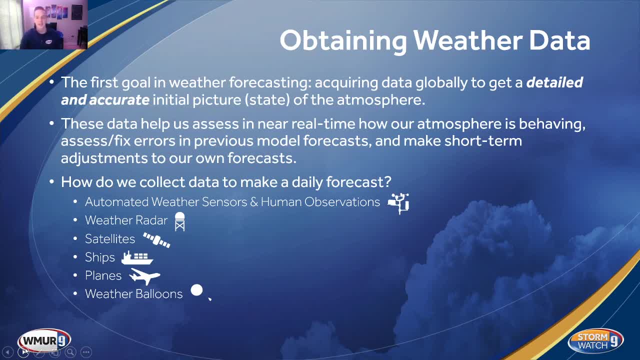 about. So we'll go through the main primary ways we collect data: Automated weather sensors and human observations- whether that be an observer saying I see a thunderstorm off in the distance or an automated sensor telling me the temperature, the wind speed and the dew point at the ground. 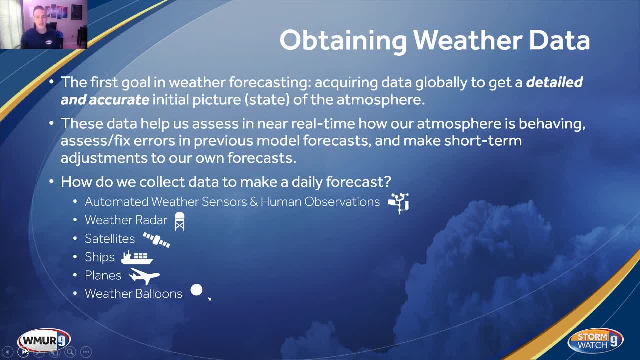 Weather radar scanning into a thunderstorm or a snowstorm, telling us whether rain or hail or the intensity of those falling. Satellites give us an idea as to how much cloud cover currently exists over space, where the water vapor is most concentrated in the atmosphere. 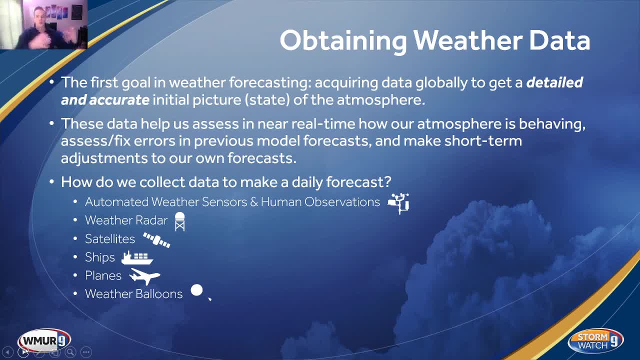 How deep, how high the clouds are, whether they have ice or just liquid droplets in them. Ships provide us crucial data over the most data sparse part of the globe, that is, our oceans, believe it or not. Planes, rather ships, help us with that, and planes to feed off of ships give us another. 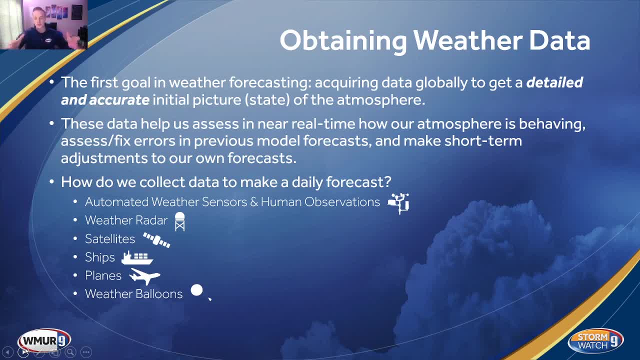 key piece of data sparse region, or allow us to see into a data sparse region way up in the atmosphere, in the jet stream, where these planes fly. we're able to collect basically key data from there. Now also note that with COVID-19 going on, we've actually lost a lot of our air travel. 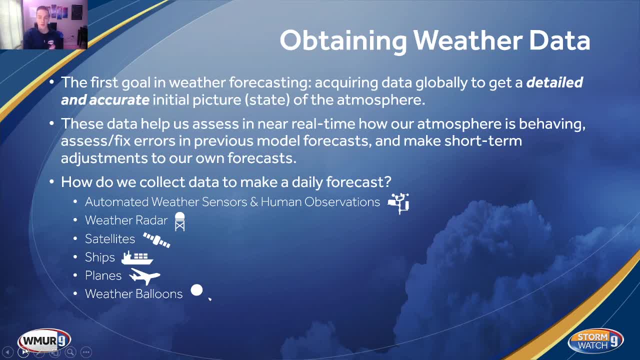 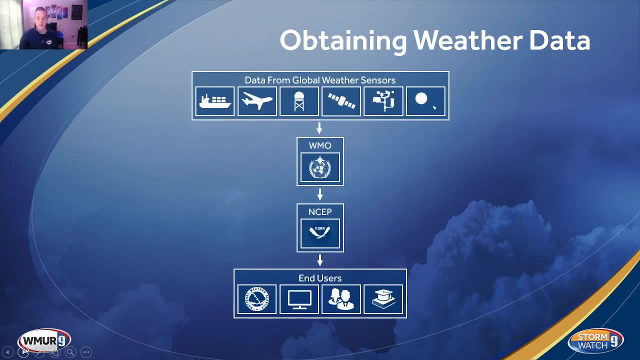 and that's negatively impacted our weather forecasts, our forecast models, because we don't have as many planes flying around. Pretty interesting to think about and one that you've probably seen a lot: weather balloons and collecting both temperature, humidity and wind speed and direction from those. 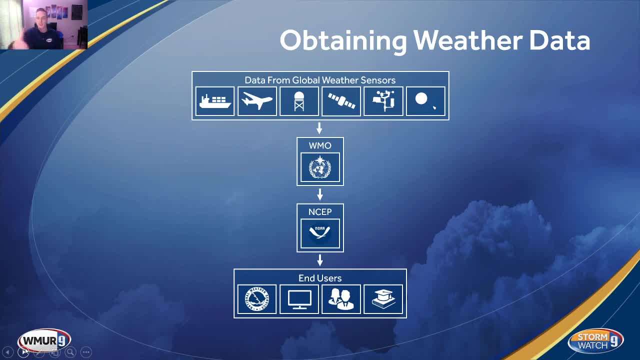 So we obtain all of our data and those six key components- there are of course a few more- and we get all this data into the WMO. they will have a strict process for both collecting for any sort of correction to the data, and then they disseminate this data to a number. 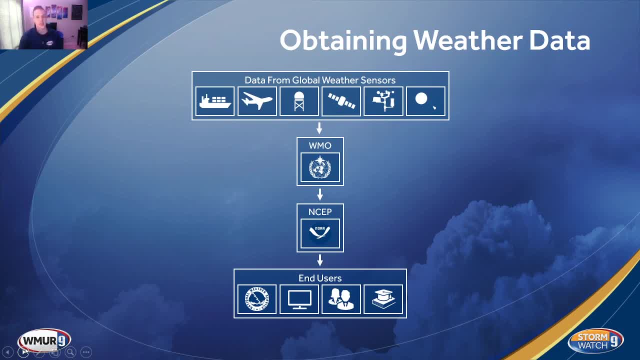 of government agencies. So in the United States we have the National Centers for Environment Prediction, housed in NOAA, and they will collect the data, they will do any additional quality control that's needed and then they will run it into their data assimilation systems and create model. 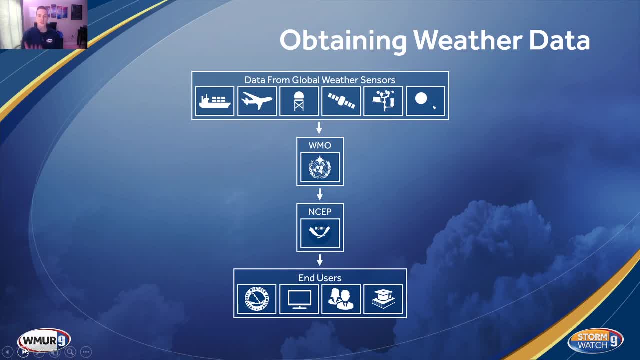 forecasts that we then, as end users, can take advantage of. We also can take advantage of that raw data as well. So some of the end users that will access this data include the National Weather Service, television- Of course- here on TV we'll use this data- private industry and, of course, academia in. 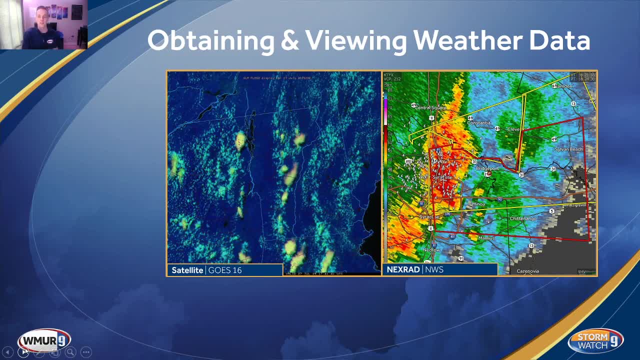 both their research capacities and some operational components as well. So here are a few ways that we will look at the data. This is a look at GOES-16. there- so the satellite image on the left- We're looking at the presence of both ice and water droplets from space and whether 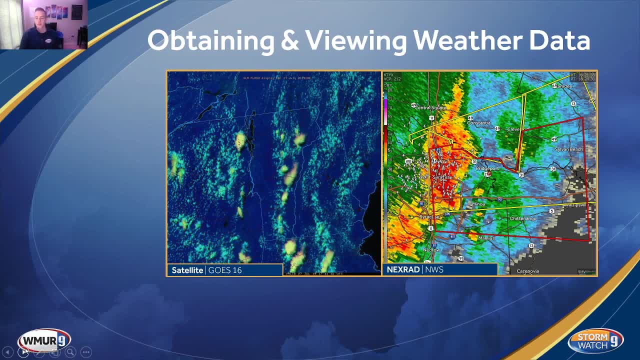 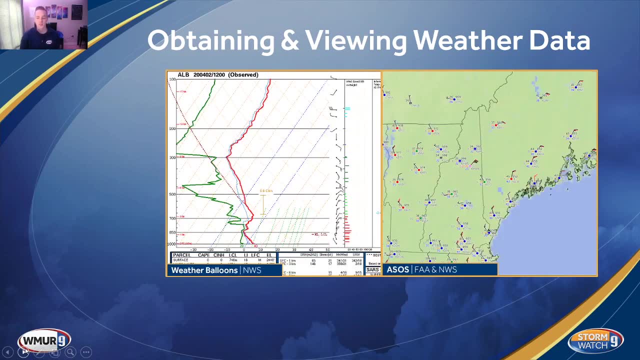 we see the onset of lightning based on a couple of other conditions there. We also can see lightning strikes from satellite Impressive. We have NEXRAD, which is the Next Generation Radar System. We have the Next Generation Radar System Run by the National Weather Service. we of course can look at radar imagery from that. 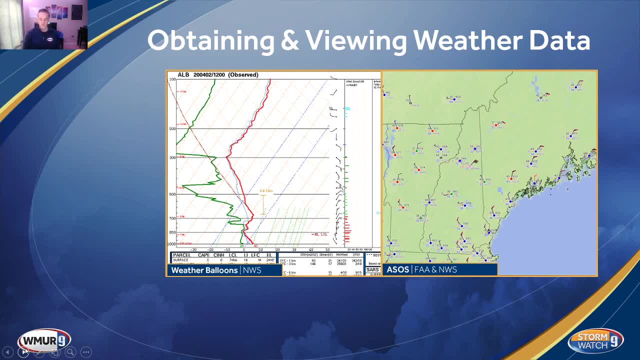 The weather balloons, imagery also provided by the Weather Service. We can plot that raw data and give us a very detailed look at both the temperature, the moisture and the wind speeds and, of course, derive other variables from those key pieces of data to tell us about the atmosphere at that launch point at that moment. 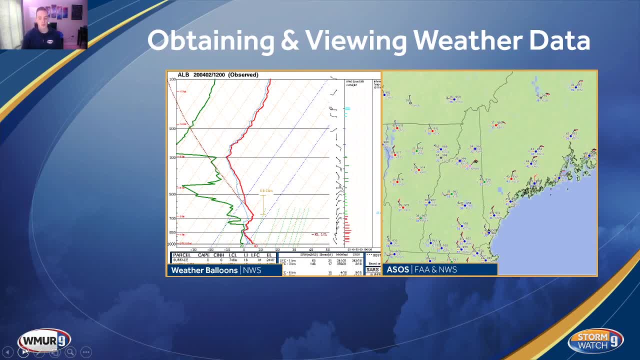 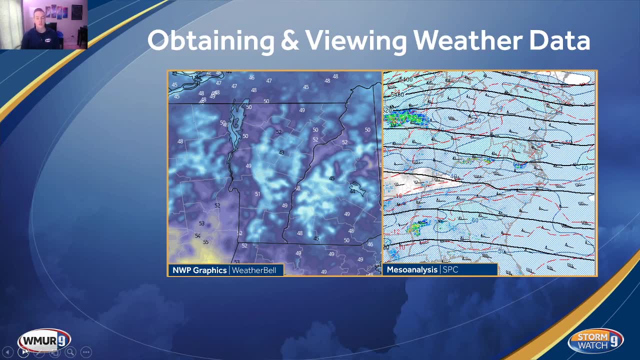 We also have the automated sensors housed in a number of airports. We have the FAA, and those allow us to see what's going on at the ground, in some cases every five minutes, which is really impressive. So our other ways we can look at data also include basically, end users, which aggregate 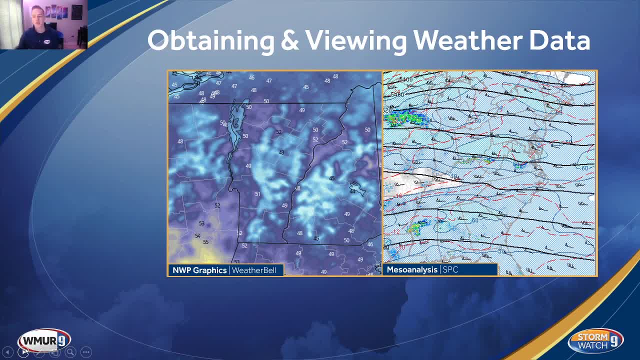 all these weather models and create model graphics for us to look at. So just a few examples, a few of the many that are out there: Weather Bell, Pivotal Weather, the College of DuPage- we have weathermodelscom. all of these sources take in this data and 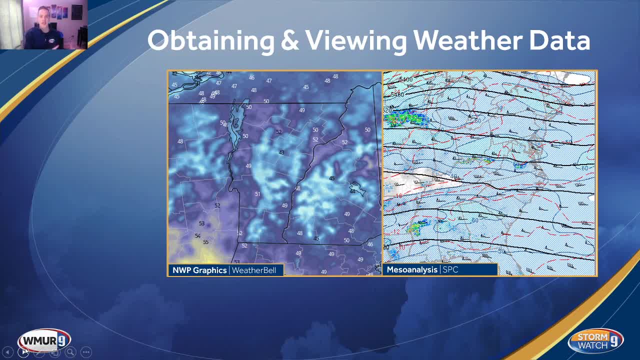 create graphics that we can use to make our forecasts every single day. Additionally the weather, we have the mesoanalysis, which is basically a near real-time weather system that allows us to see the current weather in the United States and how this looks both. 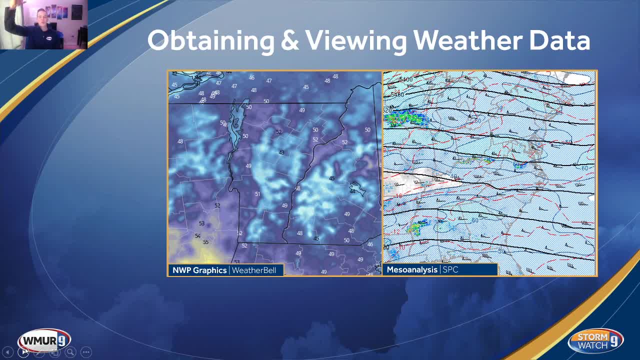 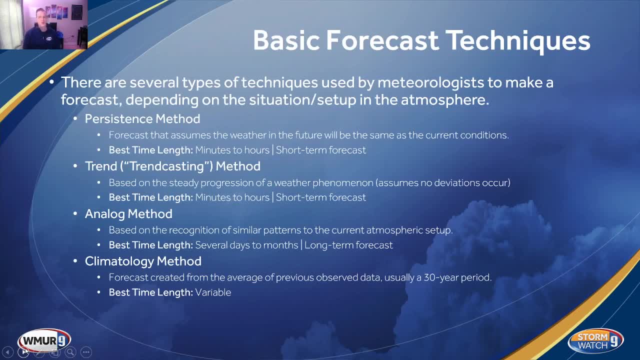 at the surface and above our heads, deeper into the atmosphere, collecting all this data and providing it into a crisp way that we can use this, and that is run by the Storm Prediction Center. So there are four basic forecasting techniques that meteorologists can take. 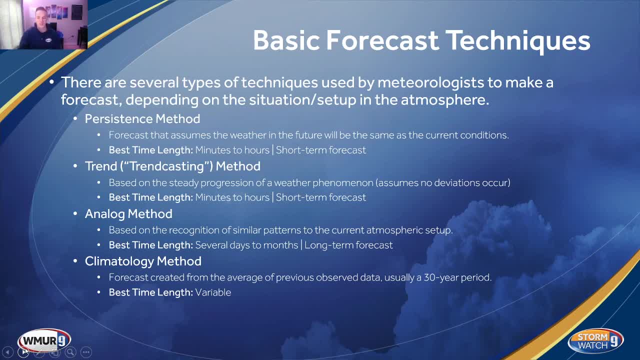 advantage of and use depending on the situation. So the first is the persistence method, which assumes the weather in the future will be the same as the current condition. So the best time length minutes to hours. an example of this would be: well, it's sunny. 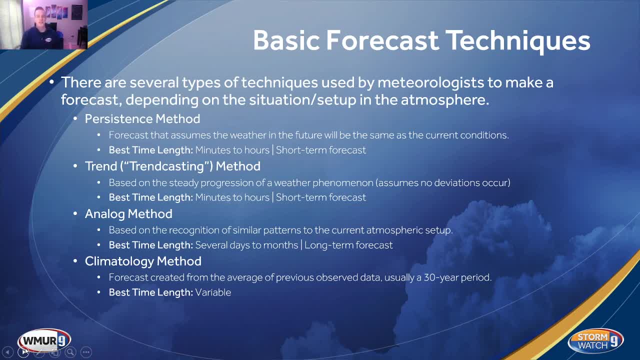 now it's going to be sunny in the future. I'm not really taking into account anything that could be changing Well, one way that this could be used in parts is: I know that the high temperature today was 65 and it was sunny. if high pressure is remaining overhead tomorrow and there's 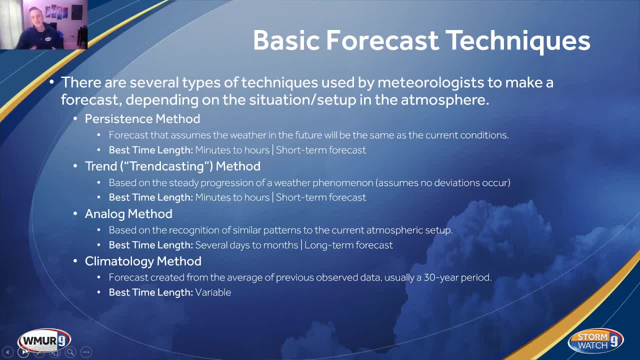 very little change in the atmosphere. It's going to be sunny and it's likely going to be closer to 65.. That is the example of a persistence forecast. Another one that's used a little more often is called a trend method or the trend casting. 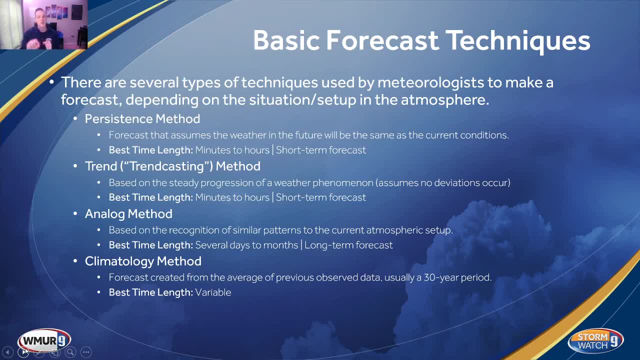 method and that's based on the study progression of a specific weather phenomenon, assuming that no other deviations to this occur. Best time length also minutes to hours. it's a short-term forecast, So we'll get into an example of that in just a moment. 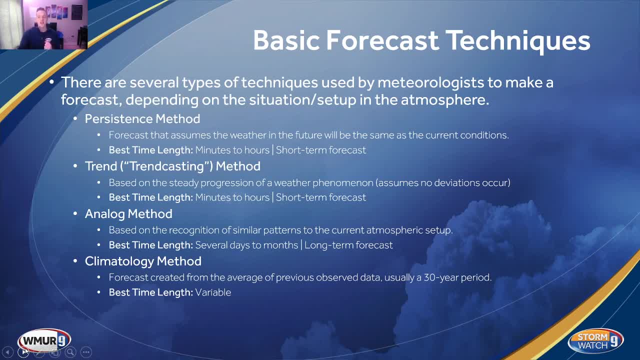 The analog method is basically pattern recognition. It's going to be a similar pattern and the conditions that it produced, and look at our current atmospheric setup compared to a pattern that's happened in the past and get an idea as to what the weather could be based on that pattern. 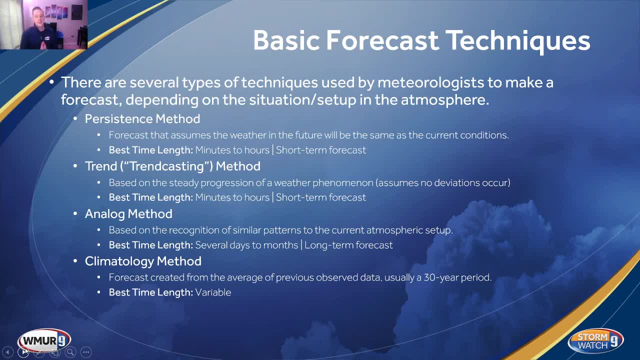 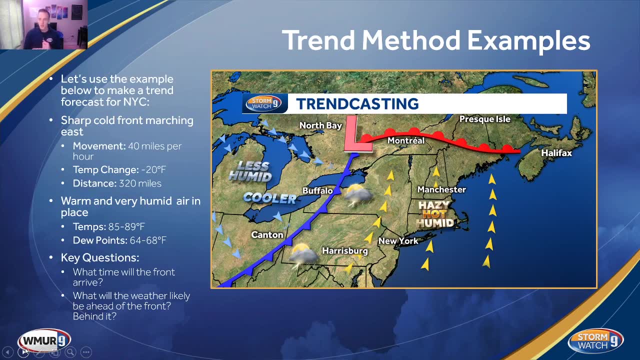 We'll talk about that in just a moment as well. And the climatology method is a forecast created from the average of previous observed data, usually a 30-year period. So let's start with the trend method or the trend casting method, and let's use an example. 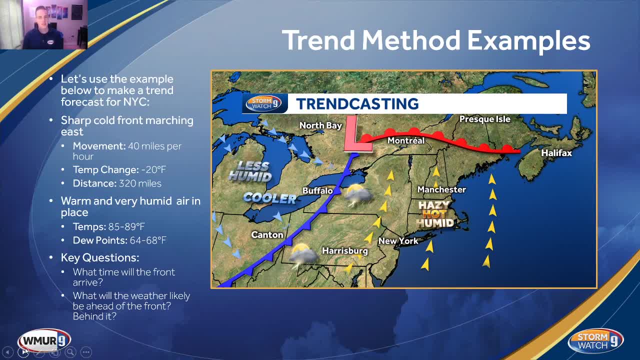 We'll use it in New York City and use the setup to basically make a trend forecast. So we know that there's a sharp cold front moving in out of the west here, out of the Great Lakes, So it's just east of Canton and Buffalo, a state of low pressure starting to march into. 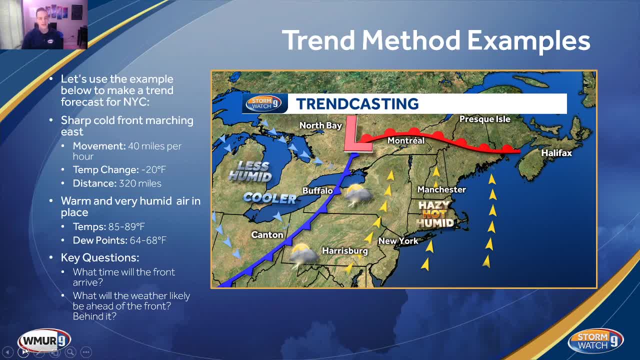 parts of Montreal and the province of Quebec in eastern Canada. It's hazy, it's hot, it's humid out, ahead of this typical summertime pattern where it's very soupy, very hot outside, perfect ingredients for some pretty strong thunderstorms. 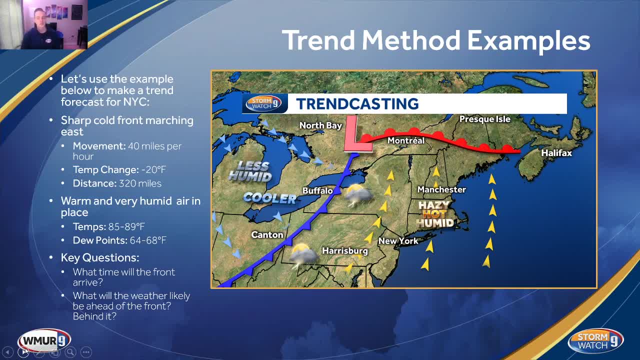 So the sharp cold front is marching east At 40 miles per hour. the change behind the front means we're going to see a change in temperature of 20 degrees Fahrenheit, but downward, And the distance from New York City to where this front is positioned is 320 miles. 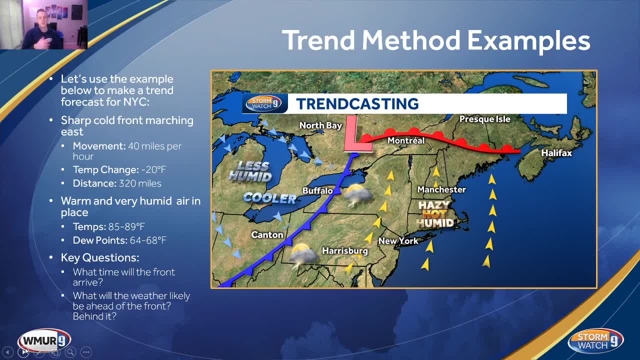 So, like I mentioned, there's warm air in place. we know our temperatures are close to 90 in some spots and our dew points are close to 70 in a few of these locations as well. So the key question: what time will the front arrive, assuming that it is moving at 40 miles? 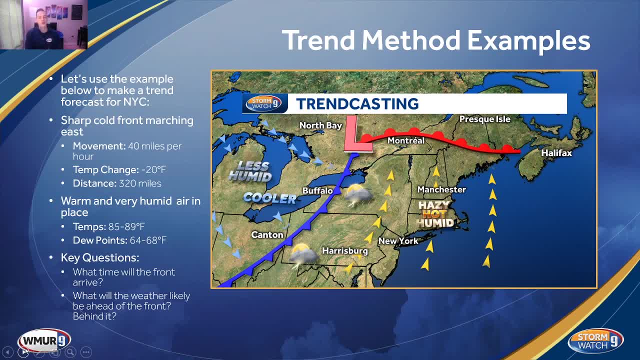 per hour at the steady state. What will the weather likely be ahead of the front and behind the front? So we know the front is 320 miles away. we know it's moving at 40 miles per hour. So in eight hours time we can expect, based on a steady trend forecast here, that it will. 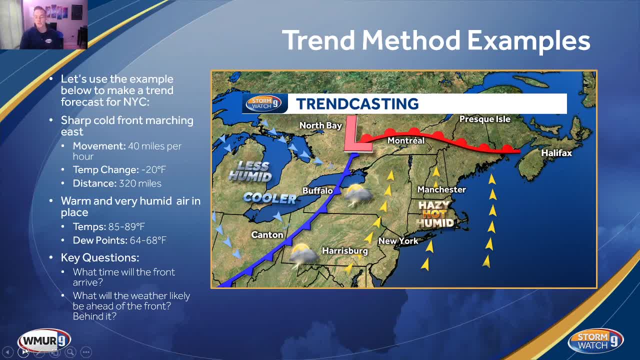 be clearing New York City, But what will the weather be like ahead of it? We know it's hazy, hot and humid, So we're going to expect sunshine to continue, it to continue to be humid, But as the front gets closer, we know that the thunderstorms will get closer as well. 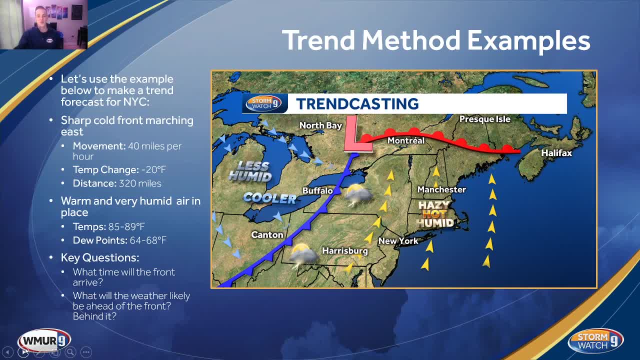 Now will the thunderstorms survive? We know that thunderstorms are fueled. They're fueled by warm, moist air in part. So of course, if that remains in place, that certainly will allow storms in part to survive, assuming other conditions are met as well and the front continues to march through. 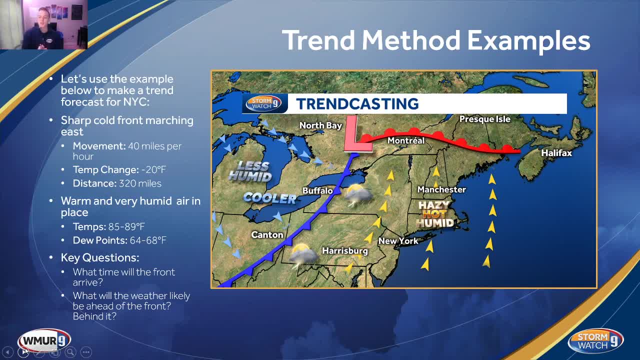 And will the forecast be behind it? Look up to the top left of the map. there we know it's less humid, it's cooler and our temperature is dropping 20 degrees. So if you look at our temperatures, subtract 20 degrees, we're talking about 65 to 69 degrees. 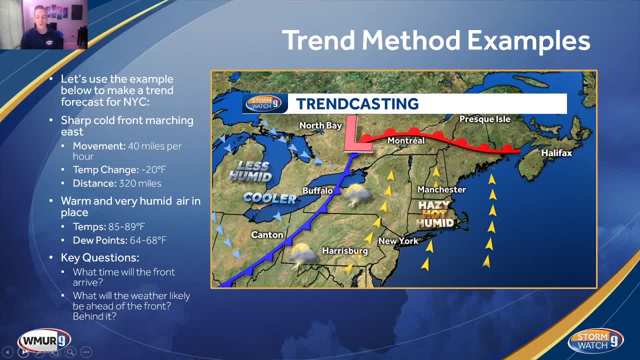 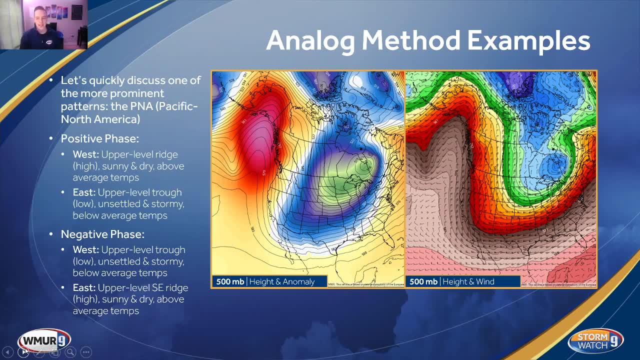 as a total drop, So we'll end up in the upper 60s When all is said and done, after the front passes. The analog method is an interesting one And one of the patterns that we look for, and occurs in the majority of months throughout. 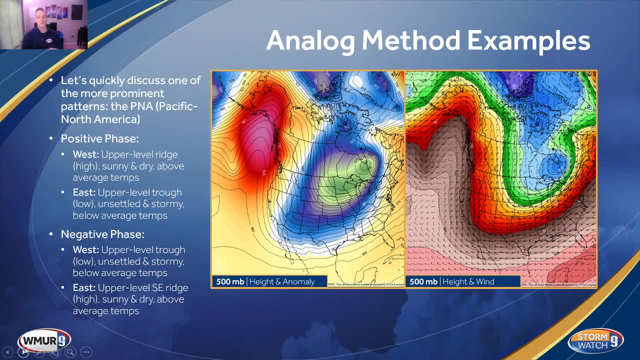 the year, only a few. where it doesn't really pop up is the P and A or the Pacific North American pattern and what that means for weather. So there are two phases to a pattern, In this case this pattern. We have a positive phase and the negative phase. 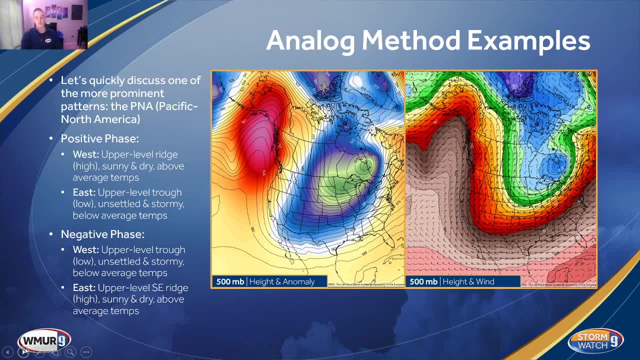 So in the Western United States and in parts of Alaska and in the South East and in the North American and in the southern states we have an upper level ridge or an area of high pressure. It's sunny and dry and we know that. 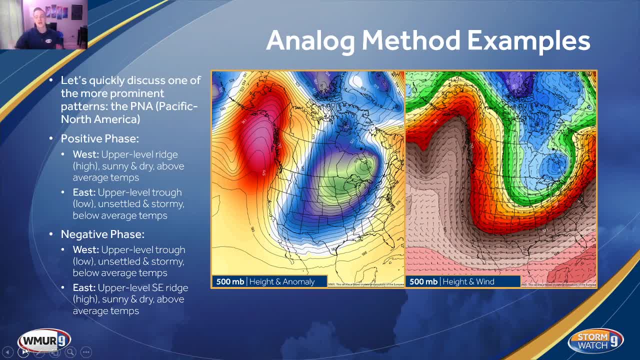 given it's sunny and dry, it's going to be above average in terms of temperatures as well. In the east upper level trough, an upper level area of low pressure continues to spiral around, So we know that it's unsettled, it's stormy, it's dragging in cooler air from the north, So we know. 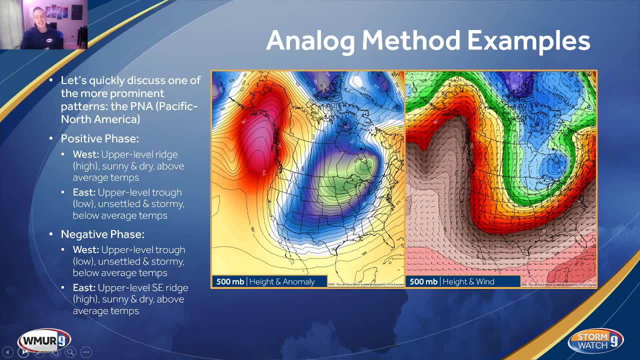 that they're going to be below average temps in this positive phase, In a negative phase. just a flip-flop of what the positive phase is. In the west we know there's an area of low pressure, stormy, unsettled, below average temperatures And in the east, high pressure. 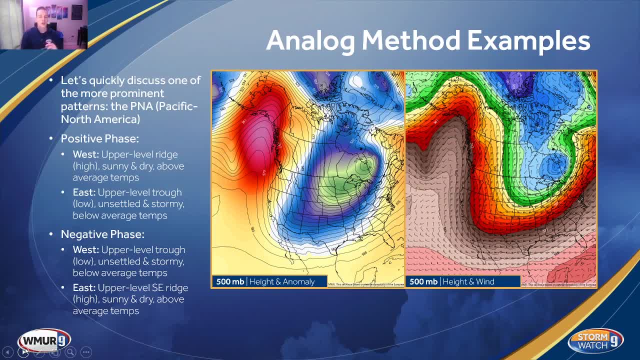 builds in across the southeastern United States. That's going to pump in hot and humid air. It's sunny and dry, above average temperatures. That region now in turn will flip to the eastern United States. So the example you see on the right is actually a forecast from the ECMWF. 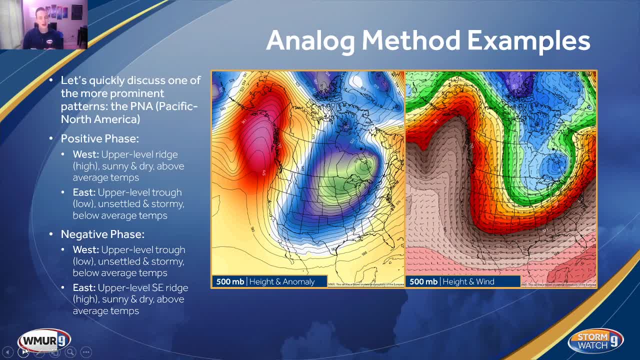 and we're looking at what is actually a positive phase of the PNA or the Pacific North American phase or the Pacific North American phase. So we're looking at what is actually a positive pattern And what we can see are basically high upper level heights across the western United. 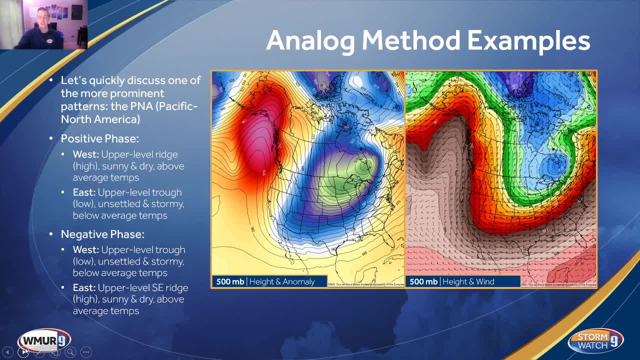 States and low upper level heights across the eastern United States. So, based on this forecast and this phase of the PNA, we can deduce the following things: just from pattern recognition, just from seeing this before, It's going to be sunny and dry in Alaska and across the west. 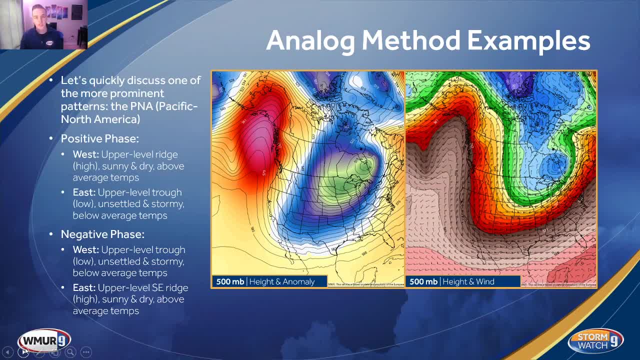 coast and parts of the west coast, and towards the east, especially just out ahead of that area of low pressure. We're expecting unsettled conditions. It's going to be rainy, It's going to be wet, Maybe we have some severe weather. in the eastern United States And we know that, in addition to that, we were getting a lobe of colder air basically moving in out of Canada. We know that there are going to be below average temperatures regardless of season, with that air mass moving in, with that pattern in place. 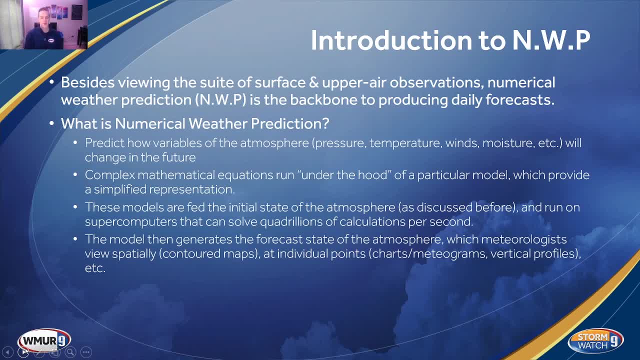 Now, any good forecaster will also use numerical weather prediction. So, besides viewing the suite of surface number observations, NWP is the backbone of our daily forecasting, day-to-day decision making. So what is numerical weather prediction? Basically, we're predicting how the 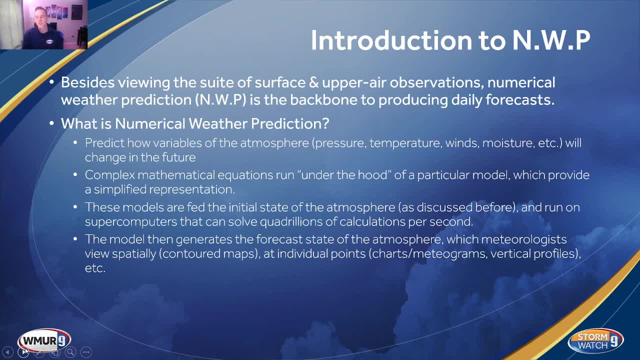 variables of the atmosphere- pressure, temperature, winds, moisture, et cetera- will change in the future. Now, this utilizes a complex set of mathematical equations run under the hood of a lot of these models- or of a particular model anyone you want to look at, which provide a 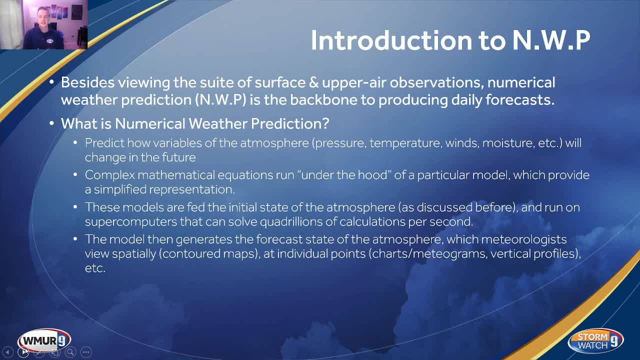 simplified representation of the weather, So we're going to use a lot of these models to predict the state of the atmosphere. These models are fed an initial state of atmospheric conditions, as we discussed before, the initial snapshot of the atmosphere, which supercomputers 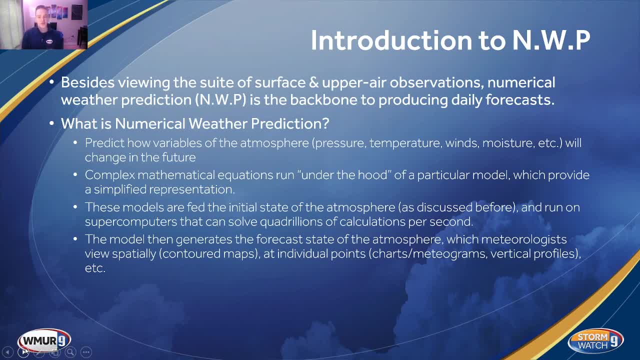 then run and can solve quadrillions- think about that- quadrillions of calculations per second to give us a forecast into the future. The model then generates the state, the forecast state of the atmosphere through time, which meteorologists will view spatially via a contour map, like you saw in a couple of slides before. 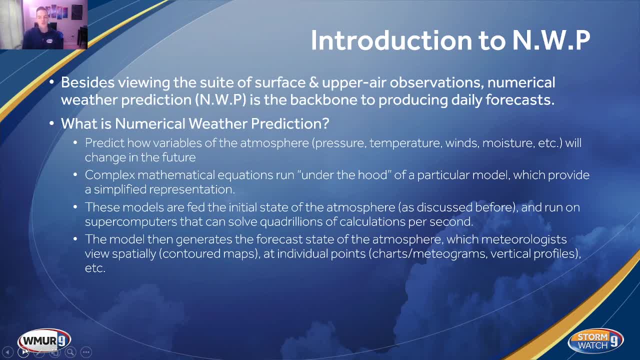 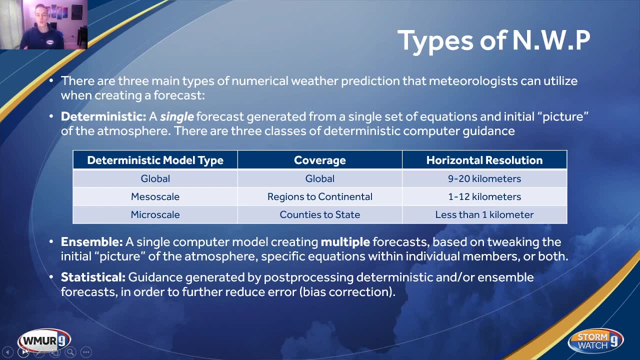 at intervals. You can see here how the waveforms are based on individual points. those are charts or media, grams, vertical profiles, et cetera. So there are three main types of numerical weather prediction that meteorologists can use on a day-to-day basis. First is deterministic. 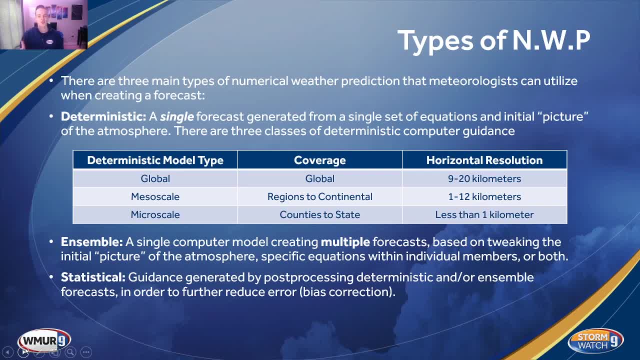 so it's a single forecast. a single forecast generated from a single set of equations and one initial picture of the atmosphere Of the deterministic models. there are three sub classes. the coverage is global and the resolution so the space in between grid points or where the model 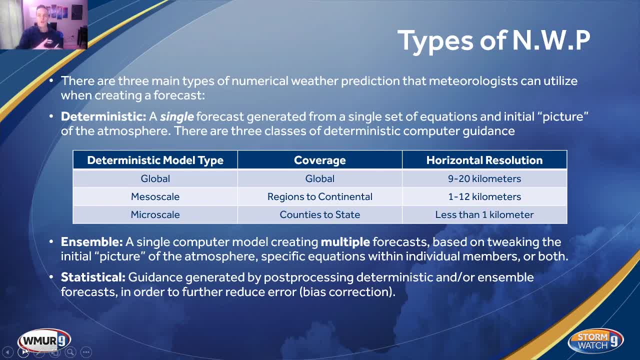 is solving for an individual point. We'll talk more about this in the next lesson. It ranges between 9 and 20 kilometers. The mesoscale is the next type. This spans from regions to perhaps a continent. in coverage It's between a resolution of 1 and 12 kilometers and some models now. 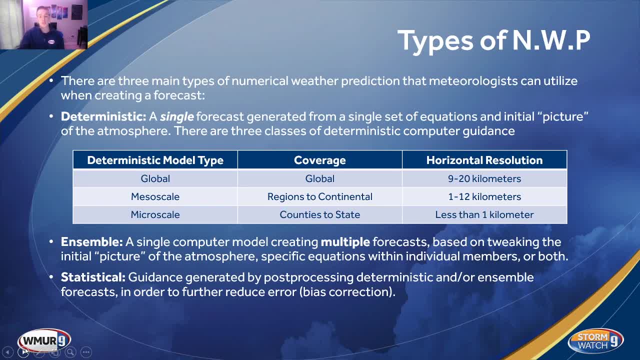 are run at the microscale, which are counties to a state level. These predict or forecast or run using past events to model things like thunderstorms or tornadoes. Those are run at less than 1 kilometer in resolution. The next main class of a model is called the ensemble model. 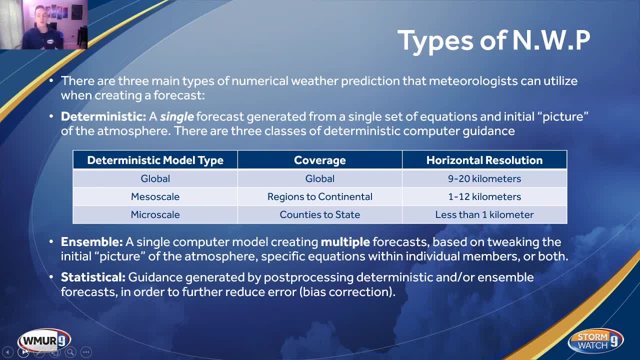 which is a single computer model creating multiple forecasts based on tweaking both the initial picture of the atmosphere specifically, and the overall picture of the atmosphere Equations within some of these individual computer models, or a combination of both. We'll talk about ensemble models in the next lesson as well. to give you an idea as to what